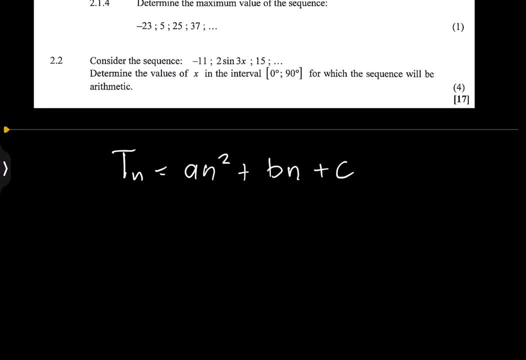 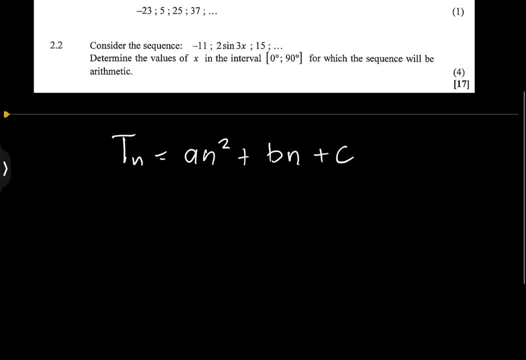 the value of Abn And C, so that we get that nth term of the expression, as they have said Right. so now, what is our sequence? So we've got our first term to be 72.. We've got 100.. We've got 120.. 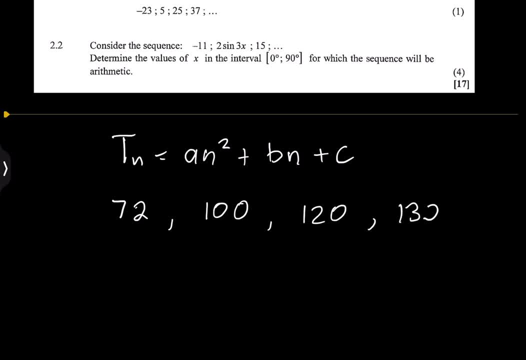 And we've got 132, I think, Okay, right. So now we find our first difference. Okay, so in this case, remember, we find the difference by taking term 2 minus term 1.. Okay so, 100 minus 72. That will. 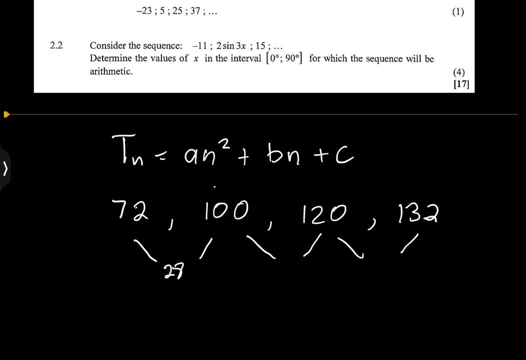 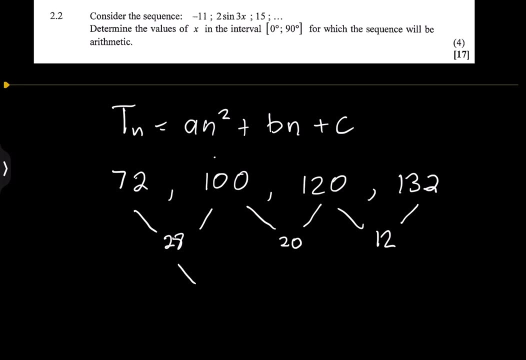 give us 28.. 120 divided by 100. That will give us 20.. Okay, and 132 subtract 120. That will give us 12.. Okay, so that's our first difference. Now, of course, we're going to try and find our second. 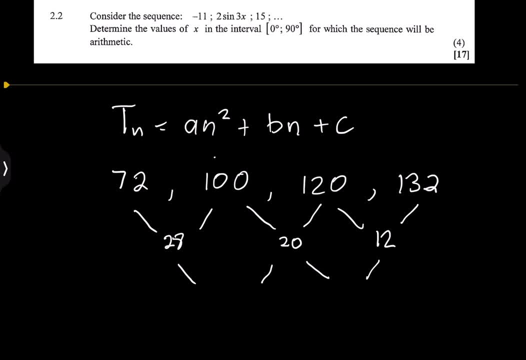 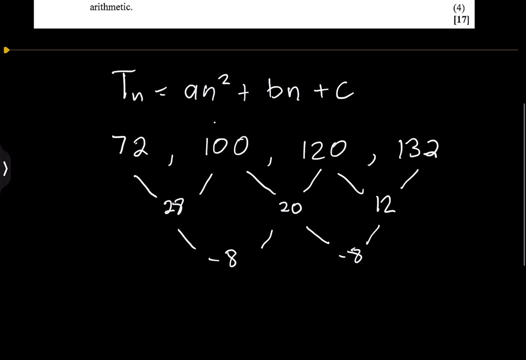 difference in this case. So we're going to say so: 20 subtract 28.. 20 minus 28 will give us negative 8.. And, of course, 12 minus 20.. That will also give us minus 8.. And remember, in our second difference, that is where we'll have a. 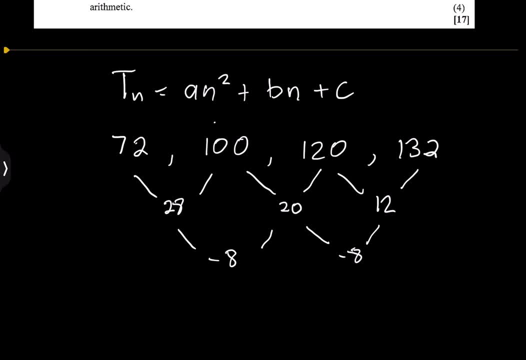 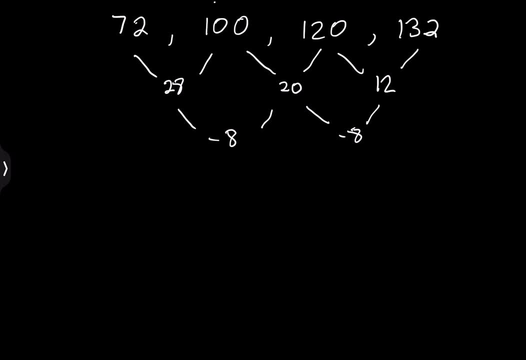 constant difference or a common difference, Right? so what we do with the arithmetic sequence, the quadratic sequence rather, is that we always now the second difference- you just simply say 2a- is equal to the value of the of your second difference. Okay, so that's equal to. 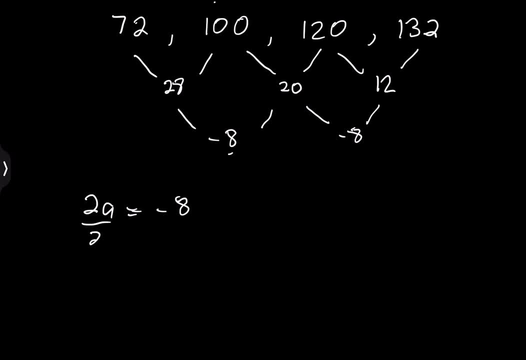 negative 8.. Okay, so to get the value of a, I'm going to just divide both sides by 2 there, And therefore a would be equal to negative 4.. Right Now, to get the value of b, what we do is that we go to the second difference, rather the first difference. So we took the 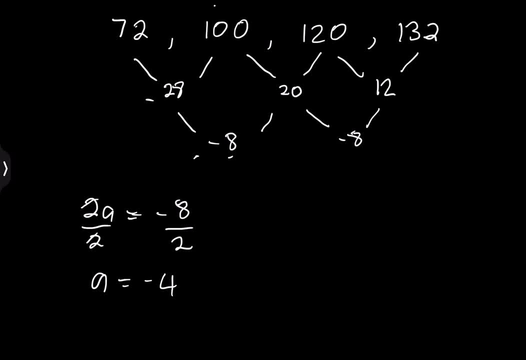 second difference and we equated it to 2a And then now remember that the first difference is simply 3a plus b. So we say this is equal to 2a, This is 3a plus b, And we know that this is going. 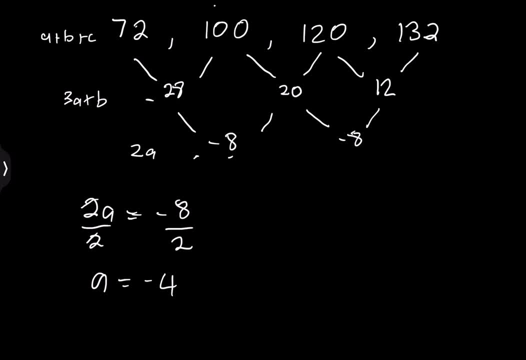 to be a plus b plus c. Okay, just keep that in mind Right. So now to find the value of b, what you're going to simply say is: 3a plus b is equal to the first term of our first difference. 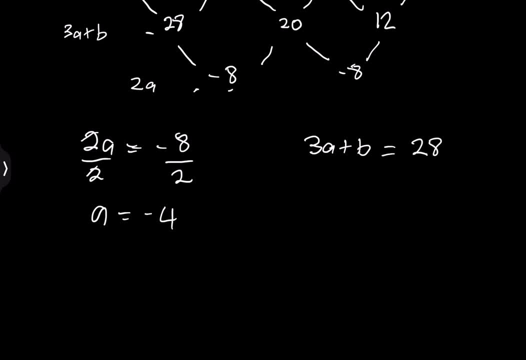 This is equal to 28.. Okay, so we know the value of b, A is already negative. 4 plus b, This is equal to 28.. And, of course, solving for this 3 times negative 4 will give us negative 12.. But if we take it to the other side, 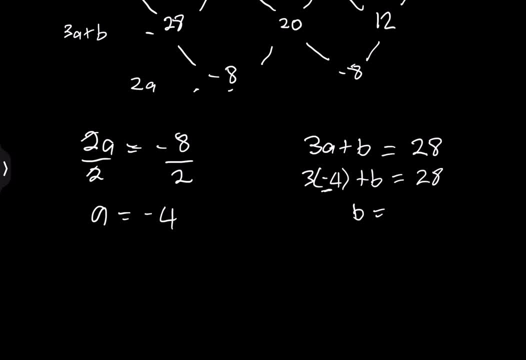 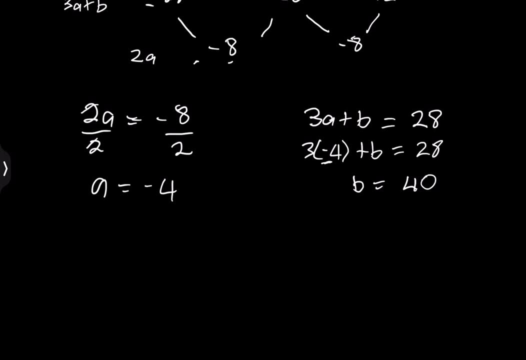 it becomes positive 12.. So in this case we've got 28 plus 12. And that will give us 40. So our b value is 40. And then, obviously, to get c, we said you go to the first term of your quadratic. 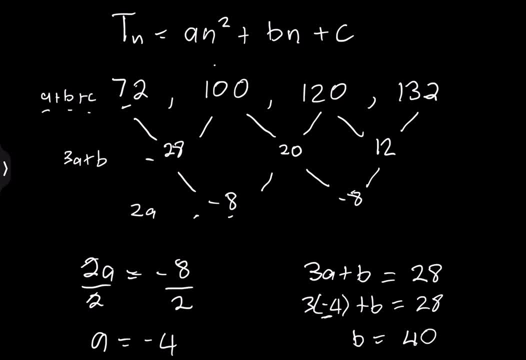 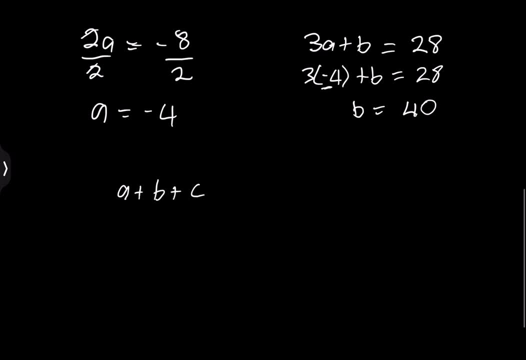 sequence And you simply say a plus b plus c will be equal to that first term. So in this case we're simply going to say a plus b plus c. I'm really not going to exhaust that much time trying to show you where this comes. 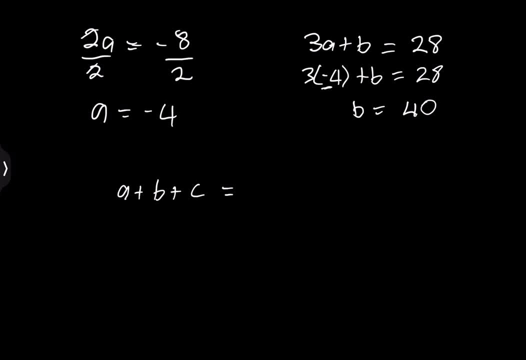 from. Of course, if you want to look at that, you're going to go into the video that we made the full lesson on this particular section, Right? So a plus b plus c equal to 72.. Okay, so I've got. 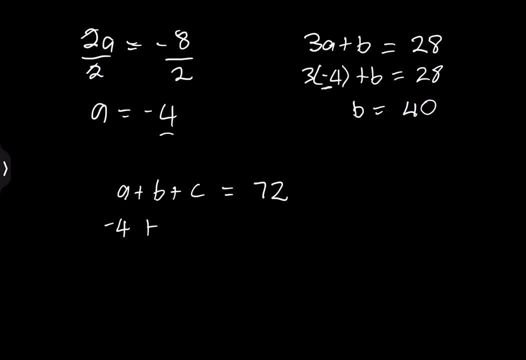 a as negative 4.. We got it there. We've got b as 40. And we've got c as we want, the value of c rather. So this is equal to 72. So in this case we've got minus 4 plus 40. In this case, that will in fact 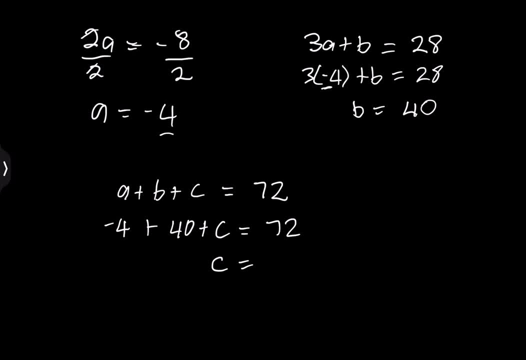 let's just take everything to the other side. So we're going to have that 72 plus 4.. So that becomes positive. Okay, so this is minus 4.. So 72 plus 4, that will give us 76 minus 40. That will give us 36.. Okay, so c is equal to 36.. 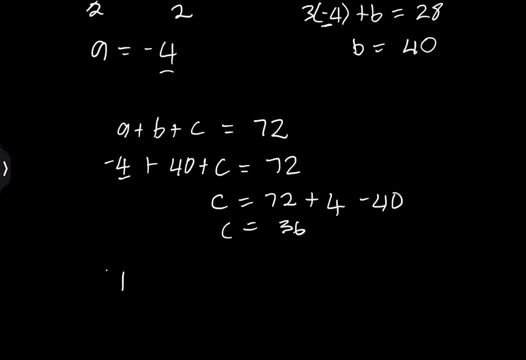 All right, Now let's write the expression in full. So it means that our nth term of this sequence is simply going to be negative: 4n squared. Okay plus 40n. Okay Plus 36.. Yeah, we've got c as positive 36.. All right, So that is our expression for our quadratic. 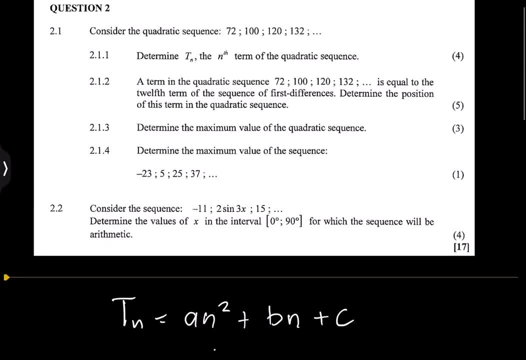 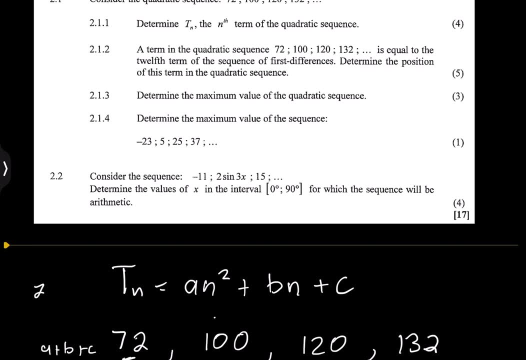 sequence. Okay, Right Now let's go to the next question. In this case, what we're going to do is look at 2.1.2.. Okay, so we answered 2.1.1.. All right, Now they say to us a term in the: 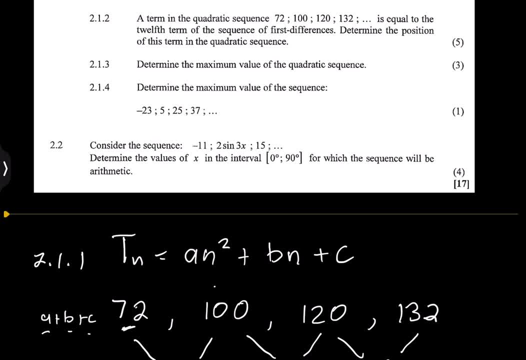 quadratic sequence is equal to the 12th term of the quadratic sequence. So we're going to do a sequence of the first difference, All right? So determine the position of this term in the quadratic sequence. Now I want you to understand very clearly, Right? So let's look at the first. 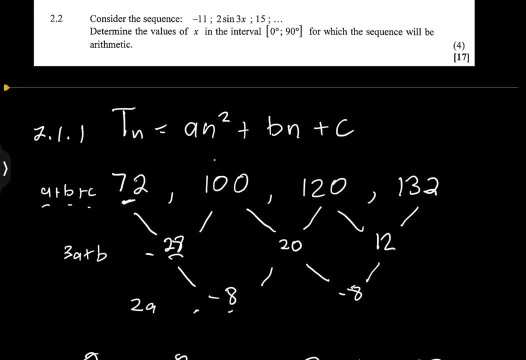 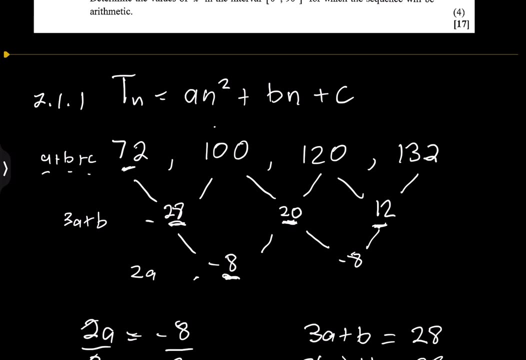 difference. So remember, our first difference is this expression here, which is 28.. So the first term is 28.. The second term is 20.. And the third term is 12.. And what is the common difference between that? it is negative eight. you remember? we got that. 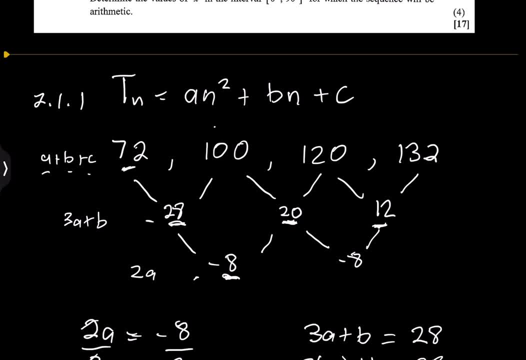 right. So in this case, what they are saying is that now, which term in the quadratic sequence will be equal to the 12th term right of this, second, of this first difference? Okay, So we need to now find what is the 12th term of that. 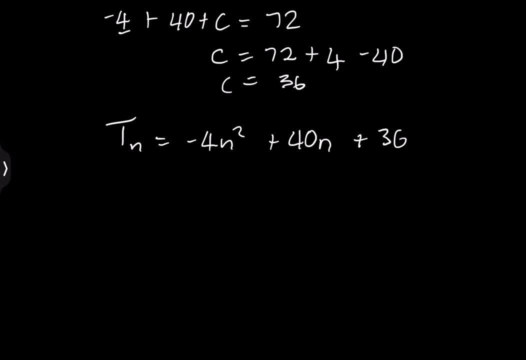 you know, first difference. So what I'm going to do is that now we're going to look at our first difference. Now you remember our sequence in the first difference. So this is 2.1.2.. So our first term in the in that sequence was 28. And then, following, 20.. And then we had 12.. Right, 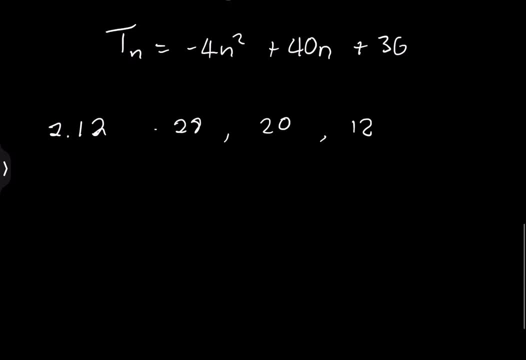 So we found the common difference to be negative eight. So that makes it an arithmetic sequence. right, because it has a common difference. Okay, And in this case, so we know that the 12th term, okay, if it's a, if it's a arithmetic sequence, we know we're going to say a plus 11 d, right? 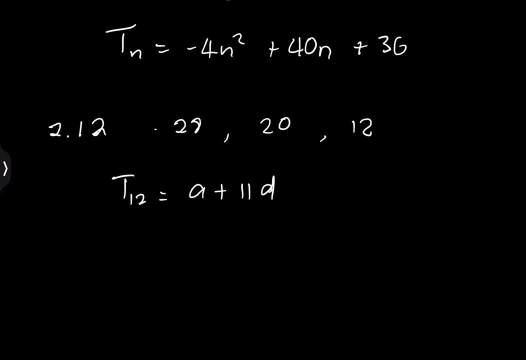 So, again, if you don't know what I'm talking about, you're going to go and look at our video on sequences and series and in particular, the arithmetic sequence, And so this is going to be a plus 11 d, Okay, 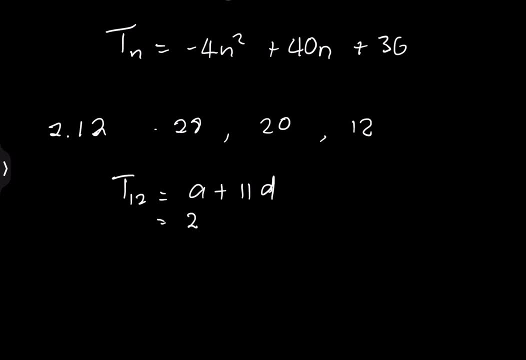 And in this case our, a value, we know, is 28.. Okay, So that's 28 plus 11 times. our common difference is negative eight, So what we actually have there, So that's 28 minus 88.. Okay, And that. 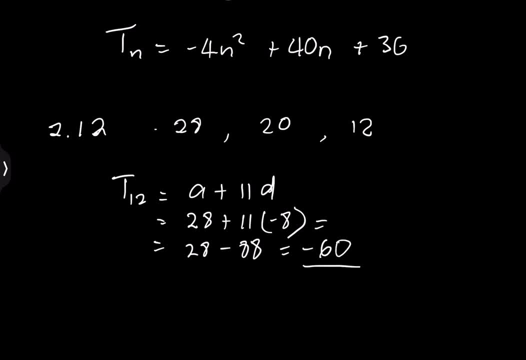 will give us negative 60.. Now we want to know in our quadratic sequence which term will be equal to minus 60.. Okay, So what you're going to do is we know in our quadratic. the expression for a quadratic sequence is negative four n squared right Plus 40, n plus 36.. Okay, and this will be equal to negative 60.. 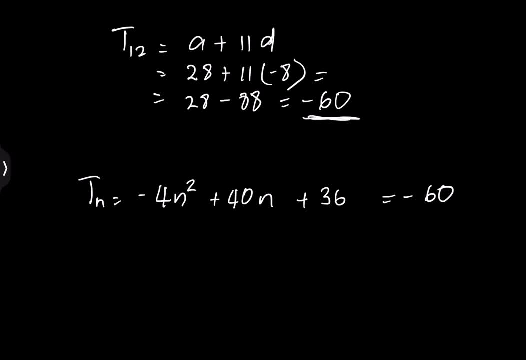 All right. So now we're going to solve that. So we're going to say minus four, n squared, plus 40, n. Okay. And then we're simply going to bring this minus 60 to the other side, so that I have a zero on the other side. Okay, so that becomes positive. So 36 plus 60, that will give us 96. And this would be equal to zero. Now, of course, let's just divide everything by negative four, Right? So if I divide this term by negative four, I'm left with n squared. Okay, and this changes to a negative. Remember, I'm dividing by negative number, So every sign changes. 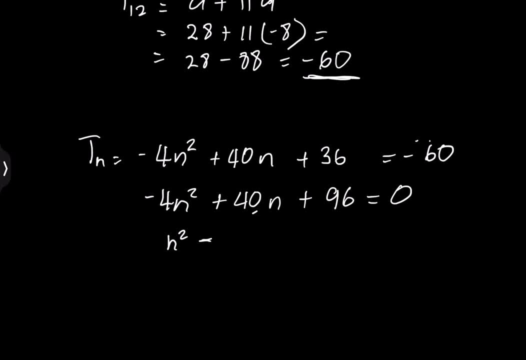 Right, So this will be 40 divided by negative four will give me a negative 10.. So that's minus 10 n And, of course, 96 divided by four, this will give me 24.. Right, But it also changes sign, So that's minus 24, which is equal to zero. Now let's try and factorize which factors of 24, which are the factors of 24 in this case, such that, when I subtract them, will give me 10.. 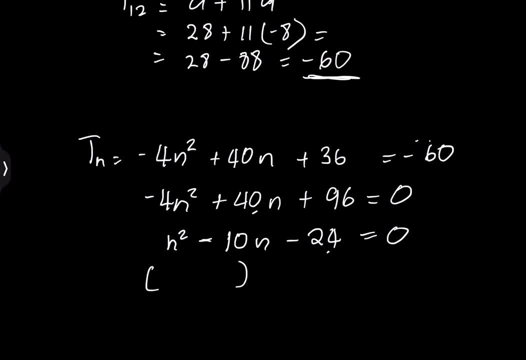 I think that will be 12 and two. So I'm going to open up two brackets there, So I'll have n and n. I'll have 12 and two. Now I want you to please note we are trying to make the middle term negative, So a bigger product will have to be negative. A bigger product is 12- n, So that means this will be negative And, of course, this will be positive. Okay, So in this case, n is negative. 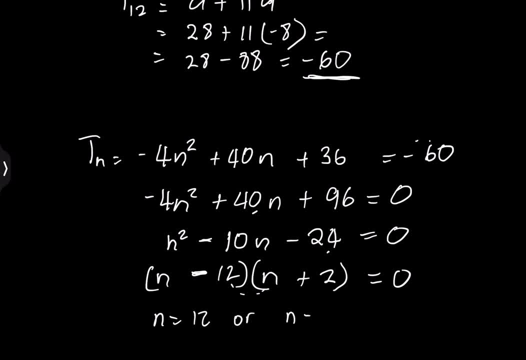 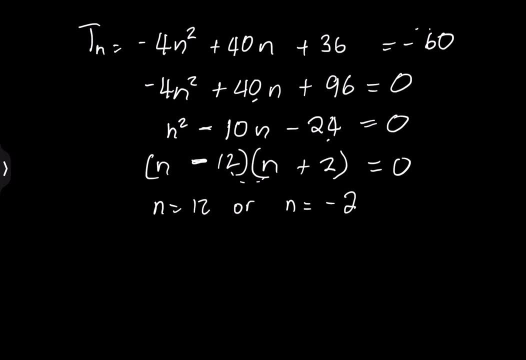 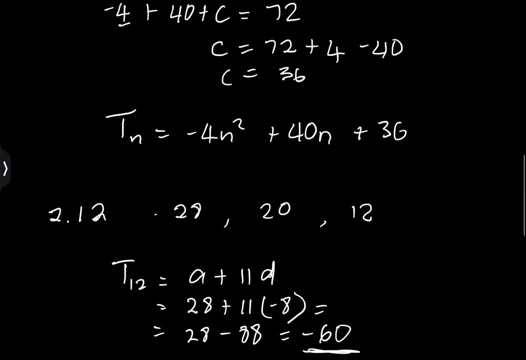 n is equal to 12 or n is equal to negative two, And of course you know this is a function of natural numbers. So it means this value will actually not be applicable. So it means that it's our 12 term that will be applicable in that case. Okay, Right, So let's continue. All right, So let me try just to move this around. 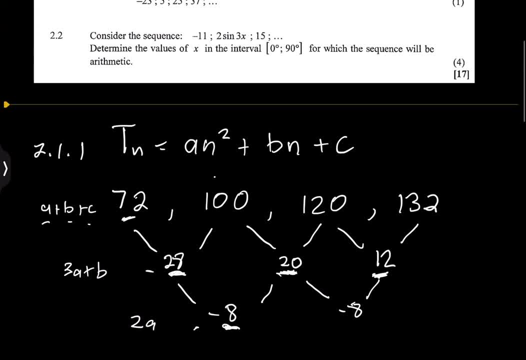 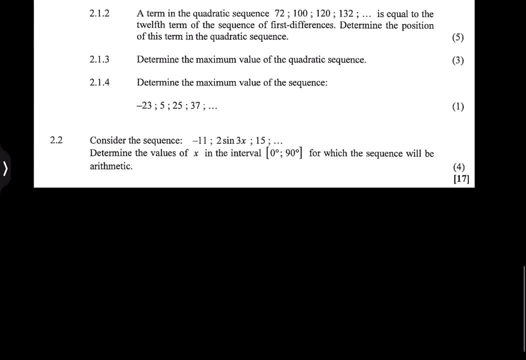 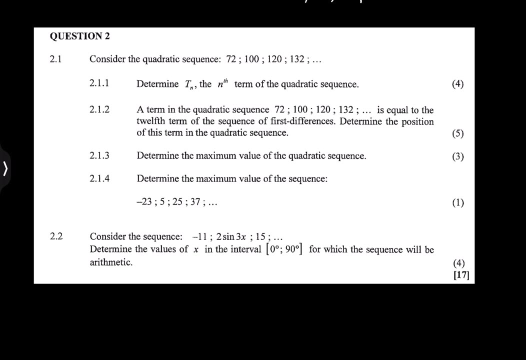 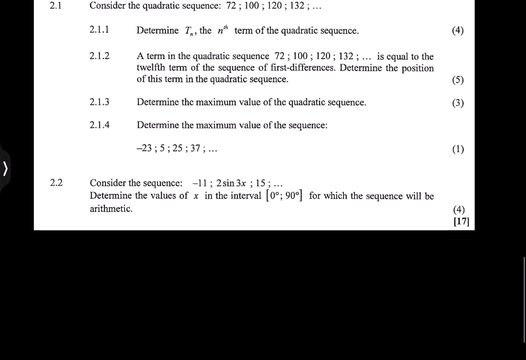 Okay, You know, I always try that you know, so that it's much easier for us to just navigate through the questions. All right, Now the next question. they said to us determine the maximum value of, you know, this quadratic sequence. Okay, So we want the maximum value. Now, remember, in this case we already have an expression for the quadratic sequence. 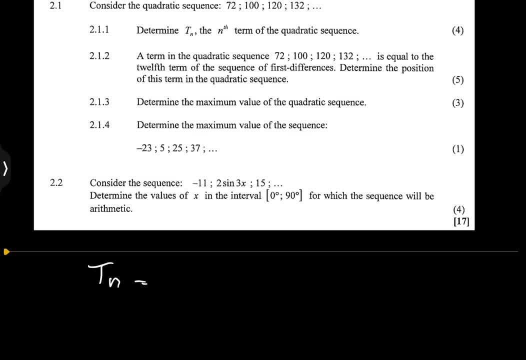 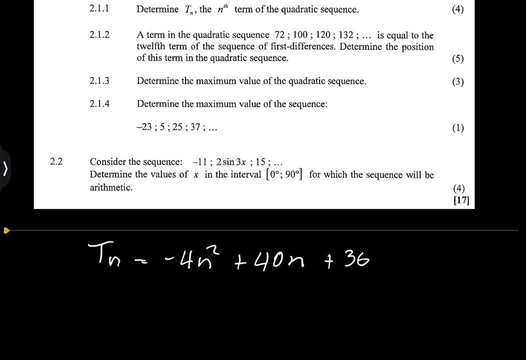 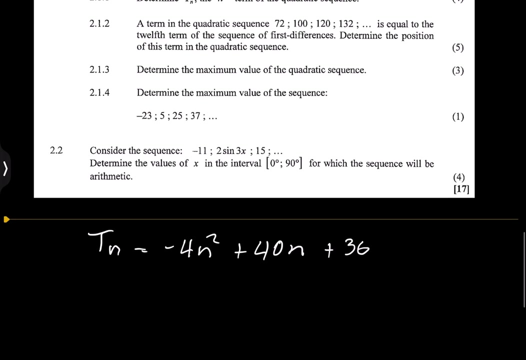 It's tn, Which is equal to minus four n squared. Okay, plus 40 n. All right, Plus 36.. Now how do we get the maximum value? I'm sure some of you are already thinking: maximum value for a parabola. What we are simply going to do is that we are going to take the derivative. Another way that we can do that is if we take minus b over n. 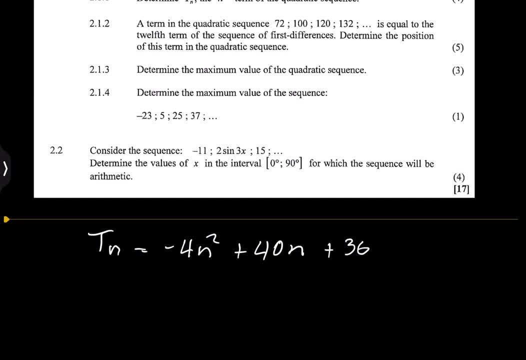 Okay, So we are going to take the derivative and make it equal to zero. So I'm going to take t dash of n, Okay, In this case. So that's our term. So that will be minus n, minus eight n. So four times two it's minus eight n plus 40. And this is equal to zero. Remember, for maximum value, we are going to take the derivative. 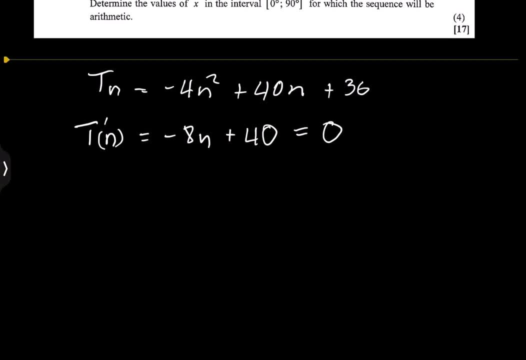 Okay, We always take the derivative and make it equal to 0. So in this case we get. so we've got. minus 8n is equal to negative 40. And if we divide both sides by negative 8, okay, our n value would simply be equal to 5.. 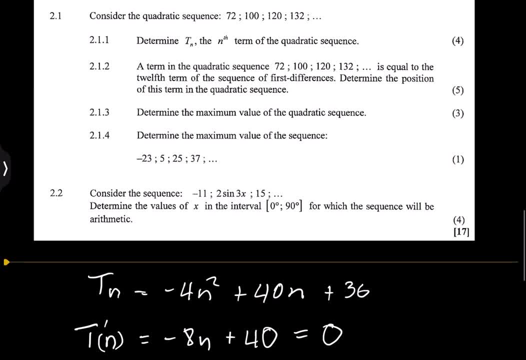 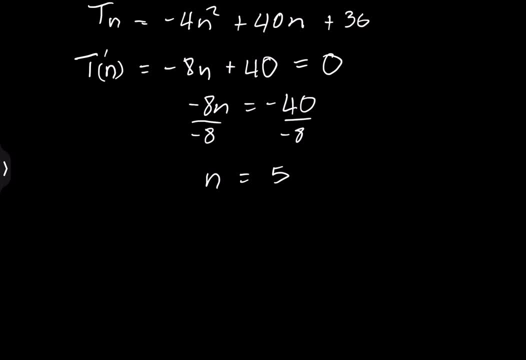 But remember, we're not looking for the term number, We're looking for the maximum value. So in this case, it means that what I'm simply going to do, I'm going to simply say: well, t5,. okay, that would be. 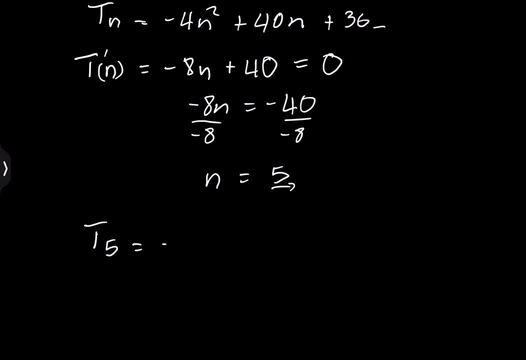 now I'm going to substitute n is equal to 5 to the original expression. So that's minus 4 times. So everywhere I see n, I'm going to put 5.. So that's 5 squared plus 40 times 5 plus 36.. 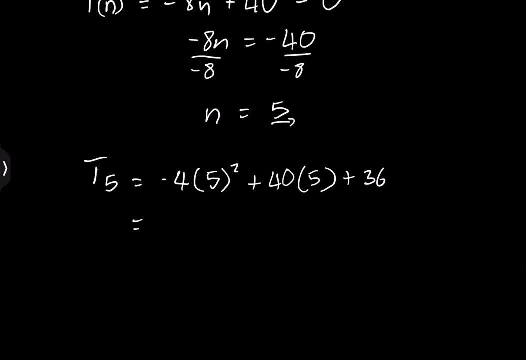 Okay, right. So in this case, what do I have? That would be minus. that's 5, squared is 25 times 4.. That would be 100.. So that would be minus 100 plus 40 times 5.. 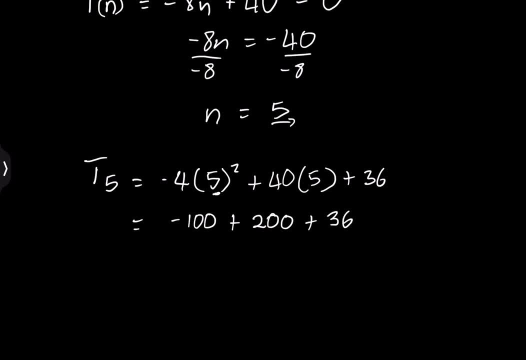 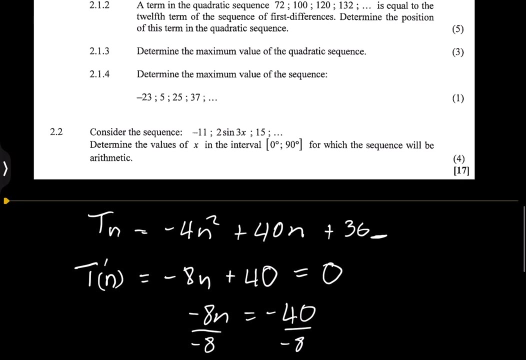 That will give us 200 plus 36. And I get a value of 136.. So obviously, in this case, it means that our maximum value in this case would be in the fifth term, which is equal to 136.. I hope that makes sense, ladies and gents. 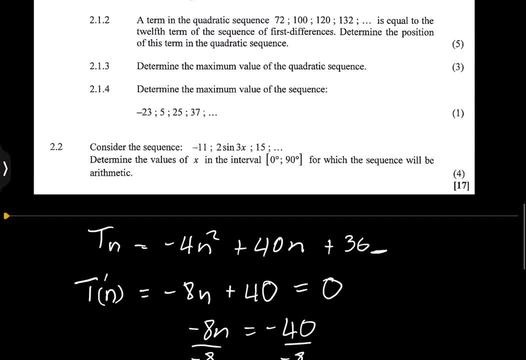 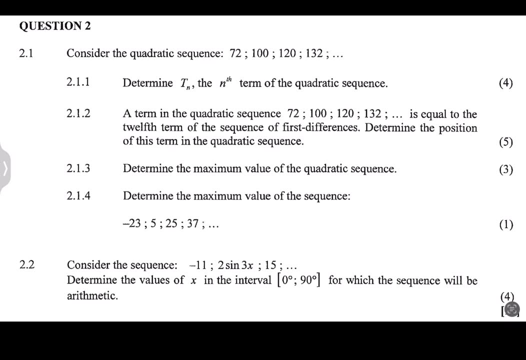 All right. Now the next question. they say to us determine the maximum value of the sequence. Okay, so they give us the sequence there. So that will be now. let me just do something here. So if you look at that sequence, let's take the- you know the constant difference there. 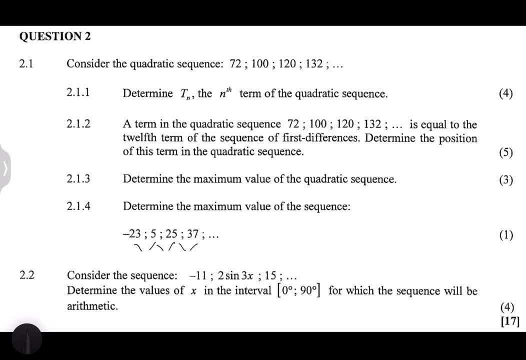 So if I say 5 minus a negative 23,, that will give me 28.. If I say 25 minus 5,, that will give us 20.. And, of course, if I say 37 minus 25, in this case, that would give me 12.. 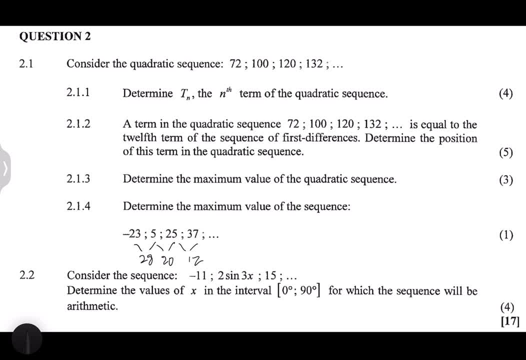 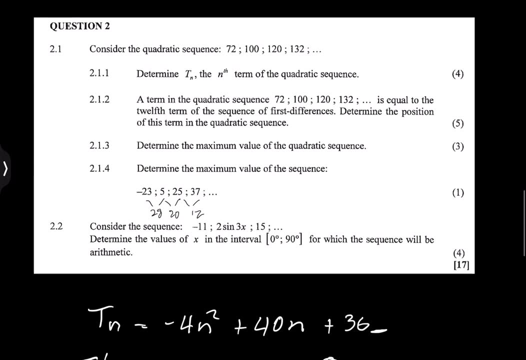 Okay, So in this case, can you see that the second difference is exactly the same as the second, or rather, the first difference is exactly the same as the first difference of our previous. you know sequence. So in this case, so once again, it's a quadratic sequence. 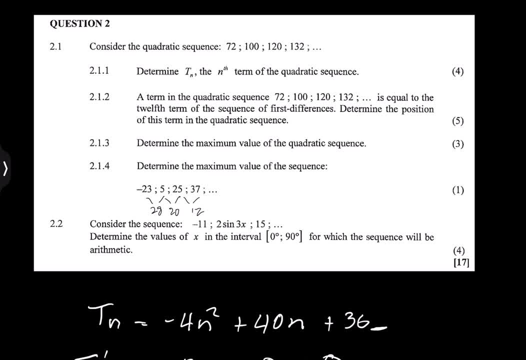 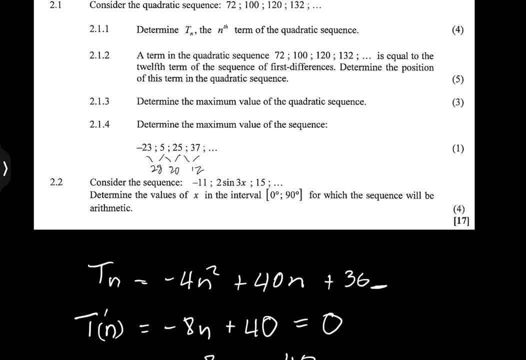 So it means that the maximum value as well will be on the fifth term, right, So what would be our fifth term in this case? I want you to please note. So if you think about the next term of the sequence now, you can see the second differences. 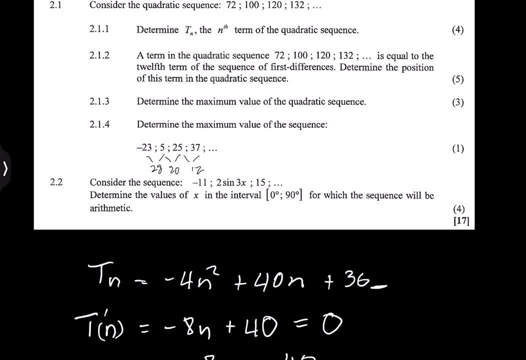 is well decreasing by eight negative eight, So meaning that the next term of your you know your, you know your, you know your your, your first difference in this case would simply be: so you'd say 12 minus eight. 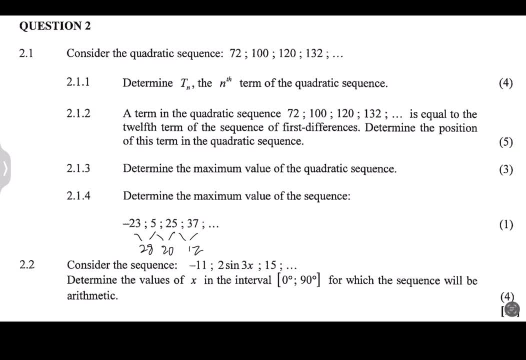 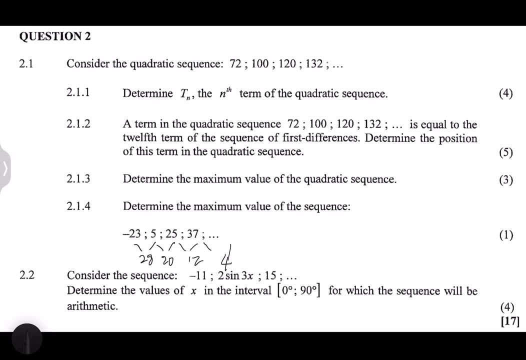 So it means that our second, or rather first, difference, the next term, would be four. So if I now want to find the fifth term right, I would simply say: okay, so we are going to take 37,. okay, So I'm going to take 37 plus four. 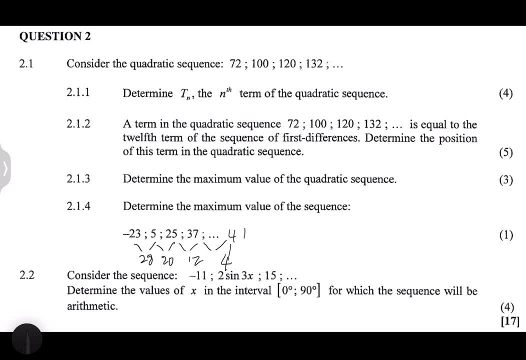 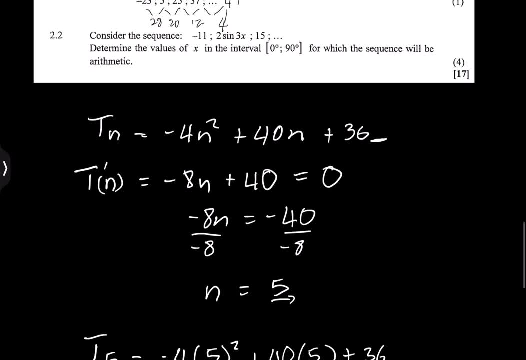 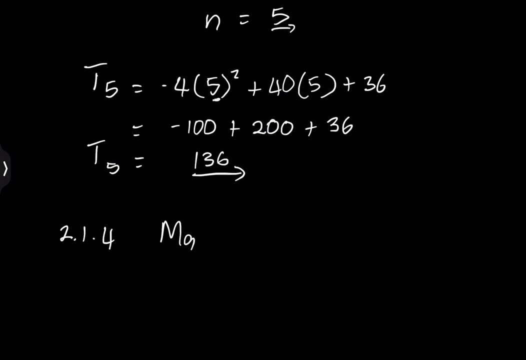 Okay, So in this case, and that will give us 41.. So that means that the maximum value so that would be 2.1.4.. So the maximum value in this case: 2.1.4.. So it means that the maximum value would be equal to 41.. 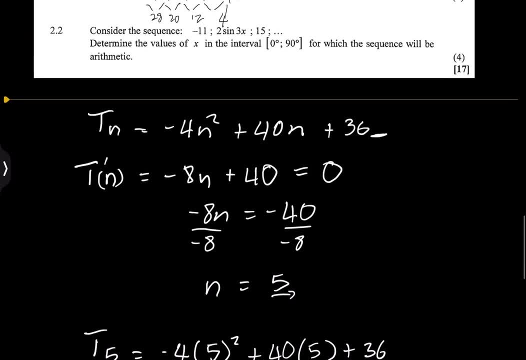 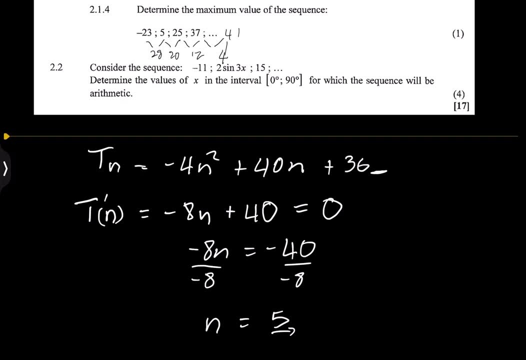 Okay, I hope that made sense. It was a one mark question, So it means that we were not really supposed to do much in terms of working out All right. Now on the last question. Okay, They say: consider the sequence negative: 11 plus two, sign three X and 15.. 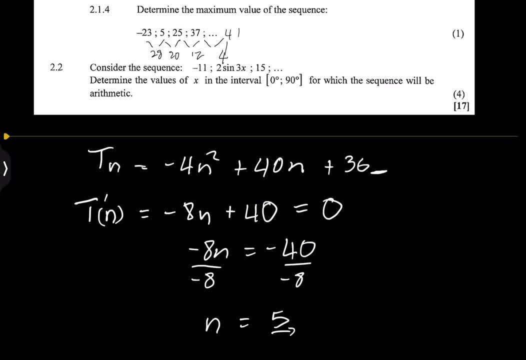 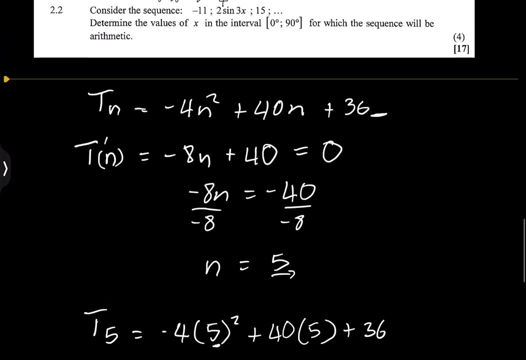 Okay, So those are the terms of the sequence. term one, term two and term three, they say, determine the value of X in the interval zero to 90, for which the sequence will be arithmetic. Now let's write down: So that's 2.1.5, right. 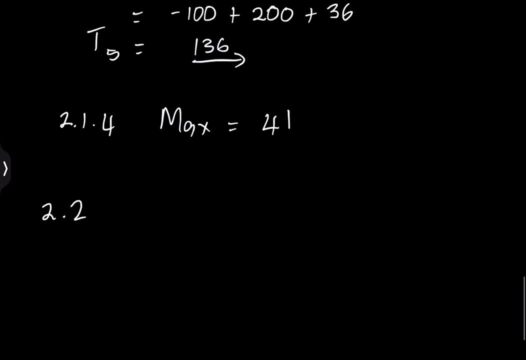 Or 2.2. actually. Okay, So that's 2.1.4.. 2. So let's now write down the terms of the sequence, Remember they said that's minus 11.. They said we've got two sign of three X and we've got 15.. 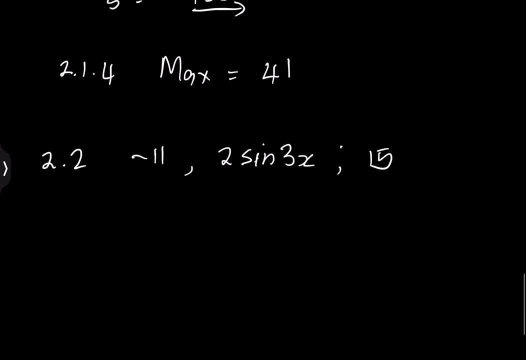 Okay. So what are we going to do? Right? Remember, they wanted it to be an arithmetic sequence, All right. So what does that mean? It means, if it's an arithmetic sequence, you know it has a common difference, right? 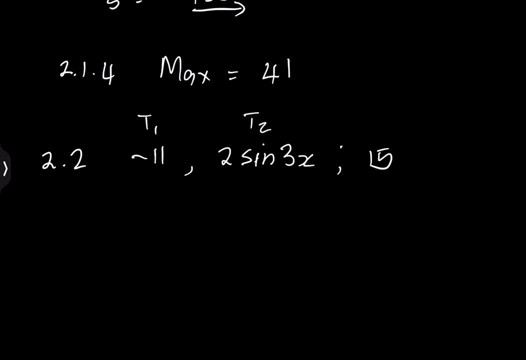 So what does that mean? So if this is term one, this is term two, this is term three. So what's going to happen is we know that term two minus term one- okay, That's what a common difference is- should be equal to term three minus term two. 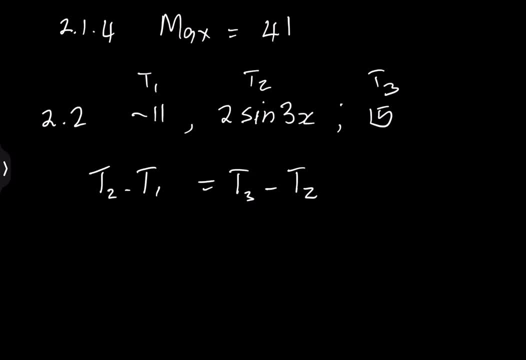 Okay, Hope that makes sense. So in this case, what is our term two? That's going to be two. sign of three: X, Okay, So that's a minus term one. So that's minus a negative 11.. Okay, And our term three? we said that's 15, okay. 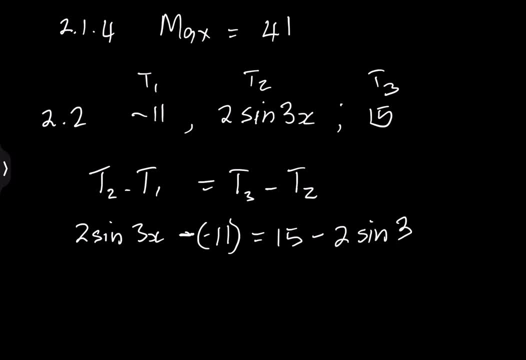 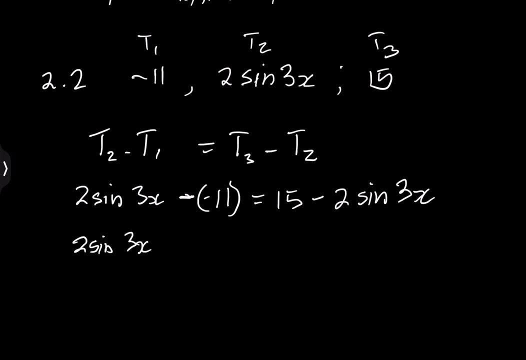 Minus two sign of three X. Okay, Right. So in this case, what do we have? We've got two sign of three X plus 11.. Okay, Remember negative times. a negative would be a positive and this would be equal to 15.. 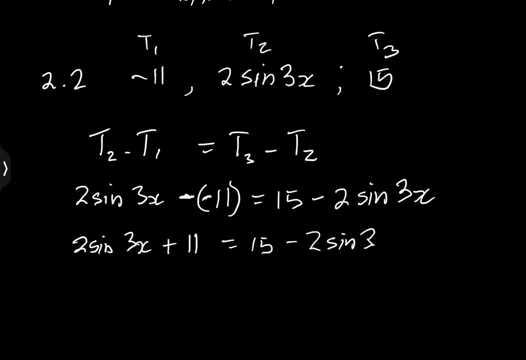 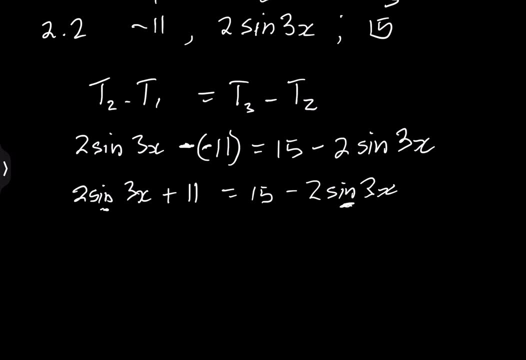 Okay, So we have 15 minus two sign of three X. Okay, Now let's group all our like terms together. So I've got two sign X. I've got minus two sign X. If I take this to the other side, it becomes positive. 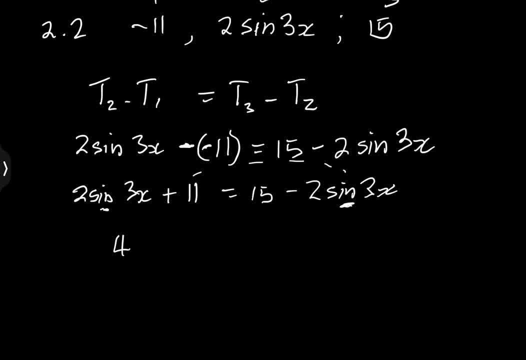 So I've got two sign three X plus two sign three X, which will be four sign of three X. Okay, And in this case I've got 15 positive. If I take the 11 to the other side, it becomes negative. 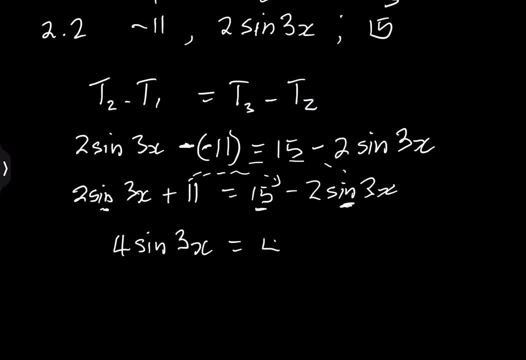 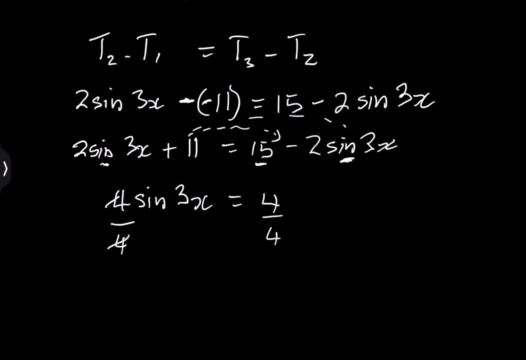 So in this case it becomes a 15 minus 11.. Which would give me four. So what I can do in this case, I can divide both sides by four. Okay, So I've got sign of three X. Okay. Four divided by four gives us one is equal to one. 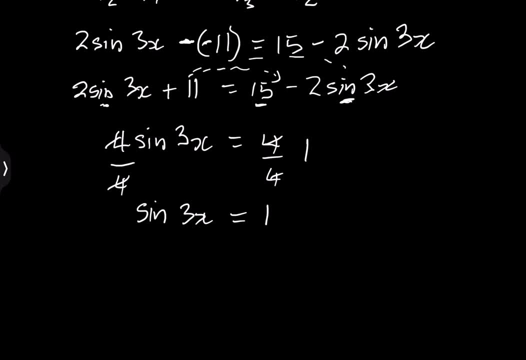 So now let's try and solve that. Okay, So we know that three X is equal to the arc sign of of one Okay, And not negative one. So arc sign of one, Okay, And in this case it means that will give us 90.. 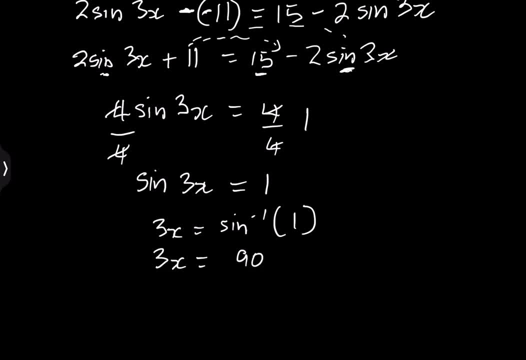 Okay, So three X is equal to 90.. Okay, Uh, but we remember, in this case, when you give a general solution, this is going to be plus K 360, okay, K 360, where K is an element of integers. but we're not looking for the general. 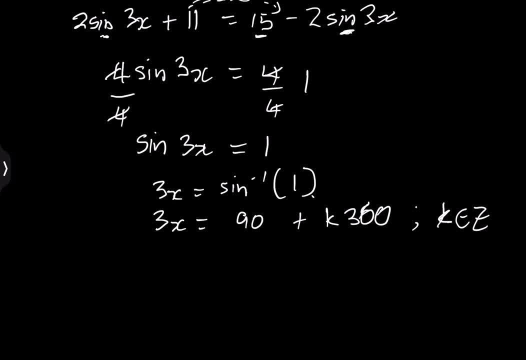 Solution: Uh, in this case we're looking for a specific. they've given us an interval between zero and 90. So we divide by three. Okay, So if we divide by three, remember we need to divide also that by three. 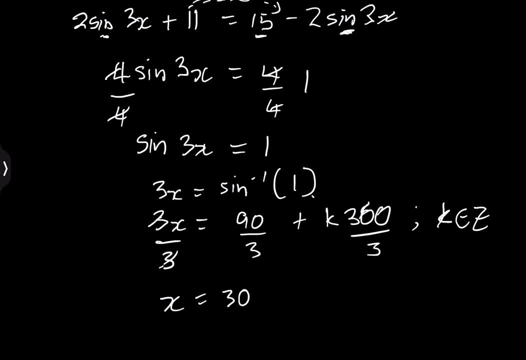 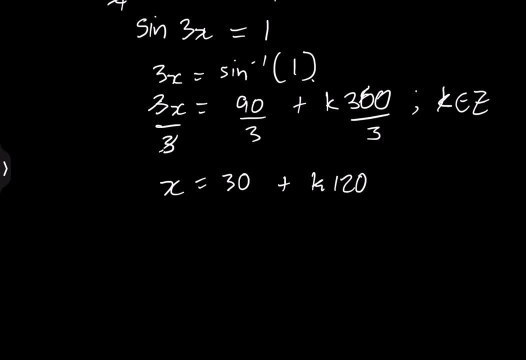 Okay, So it means that X is equal to 30.. Okay, Plus K: 120.. Okay, So that is our solution. However, in this case, because they've given us an interval, We need a specific value for X, Right? 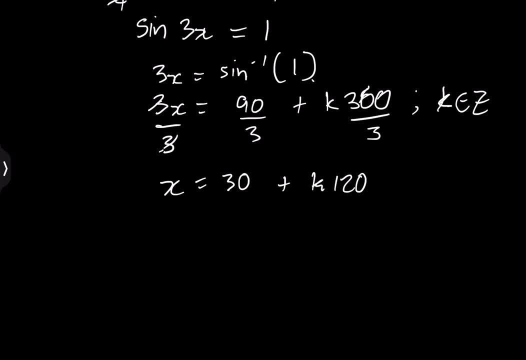 Uh, we're not looking for the general solution, but a specific value for X. So, in this case, what will fit? the risk? the restriction? uh, zero to 90.. And, by the way, uh, if you said one 80 minus 90, which? uh, of course, this is um uh. 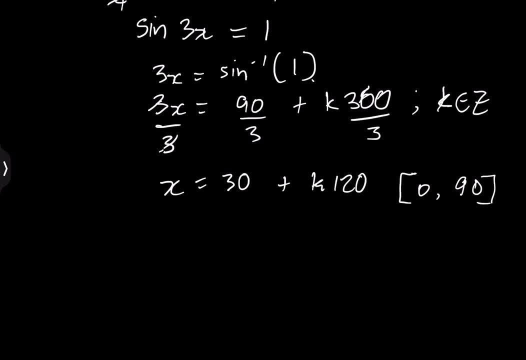 you know, sign you always give the reference angle and one 80 minus that reference angle, And in this case you would have still got in 90. So that's why I didn't bother much with it. Okay, So, um, what I'm going to do is okay. so there's nothing that we can substitute here. 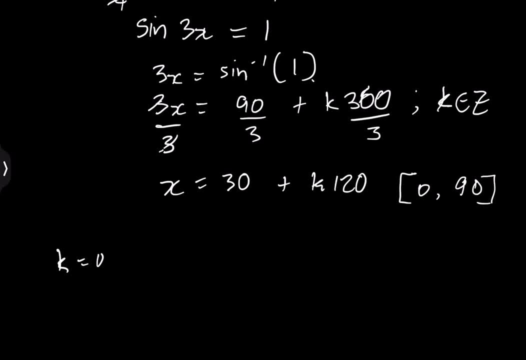 So if we say K is equals to zero, um, K is equal to zero. So we've got: uh, X is equal to 30 plus zero times one, 20.. Okay, So does that fit the restriction? So our answer is equal to 30.. 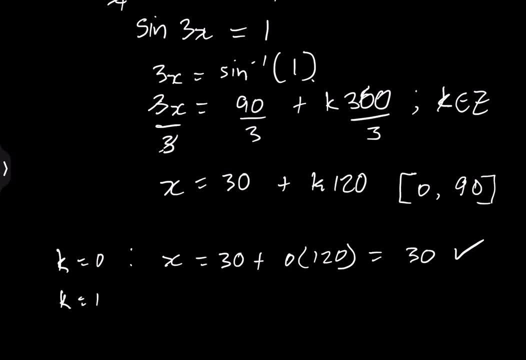 Okay, That works. If we say: K is equal to one, Okay, Uh, X is equal to 30 plus one times one, 20.. Okay, So now that would give you 150. that is outside of that restriction that you are given. 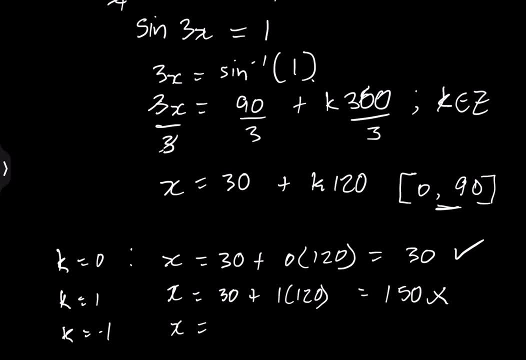 And if we also use K is negative one. So X would be equal to 30,. all right, um plus um, so that would be negative one times one, 20.. Okay, And in this case, uh, what you would get there is negative. 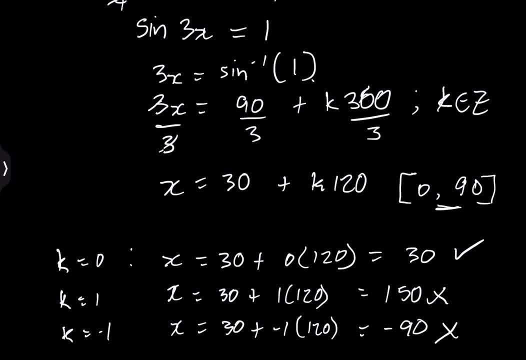 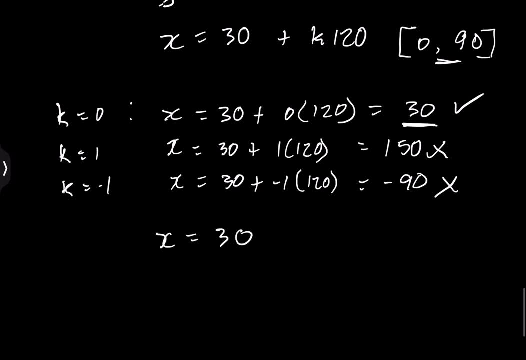 Okay, So that would be 90. And of course that does not fit the restriction, So it means the only solution that we have there, uh, is X is equal to 30.. All right, ladies and gents, I hope that made sense.